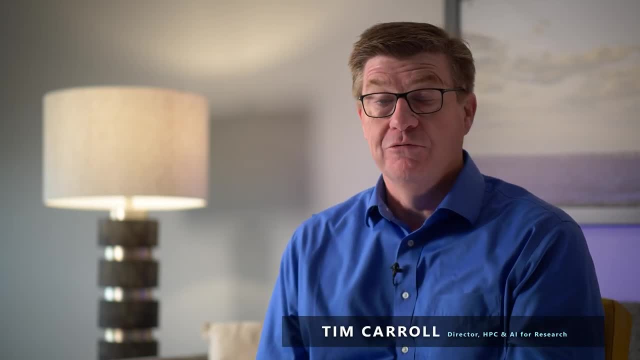 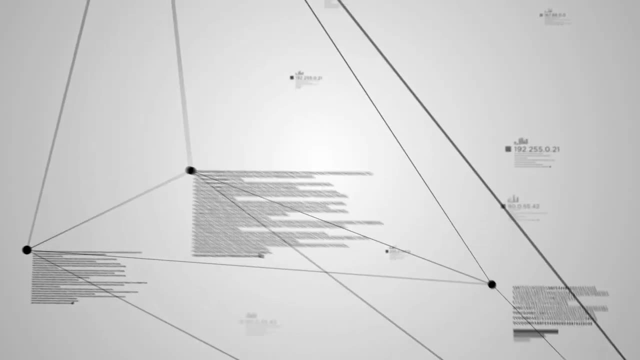 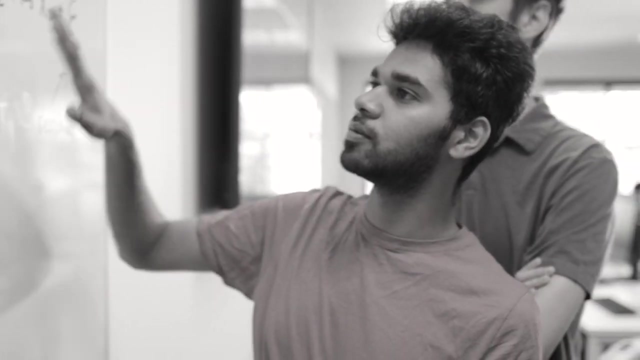 I'm Tim Carroll. I lead Microsoft's efforts to support the global research community. What is HPC? HPC is High Performance Computing, But if we go back 100 years ago, computers were actually people. The early physicists realized that if they could put more computers 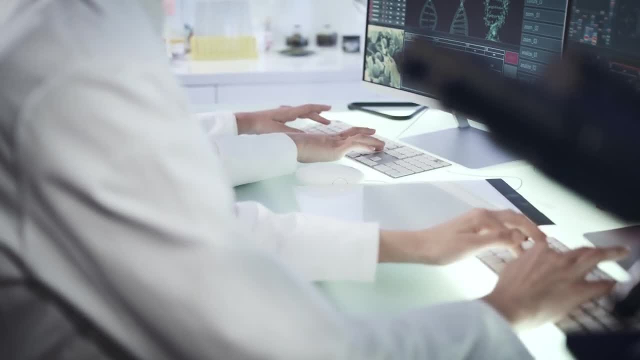 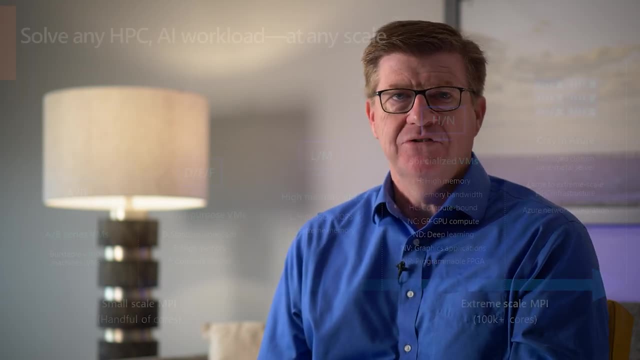 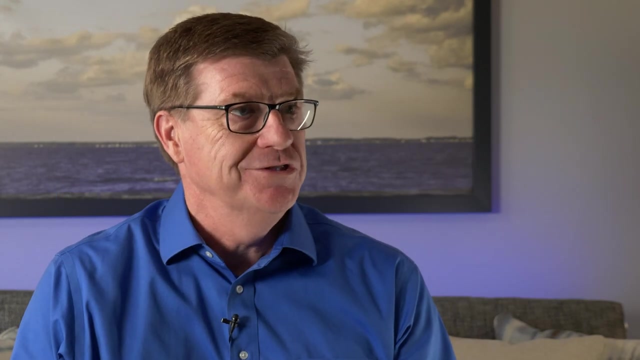 or people onto a single problem, they could get the answers faster. Fast forward to where we are today, and if one computer can solve a problem, 5,000 computers can solve it even faster. That is HPC. I've been doing this for almost 20 years now, and what has been? 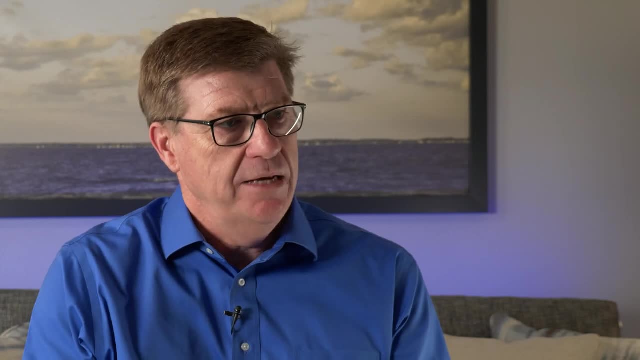 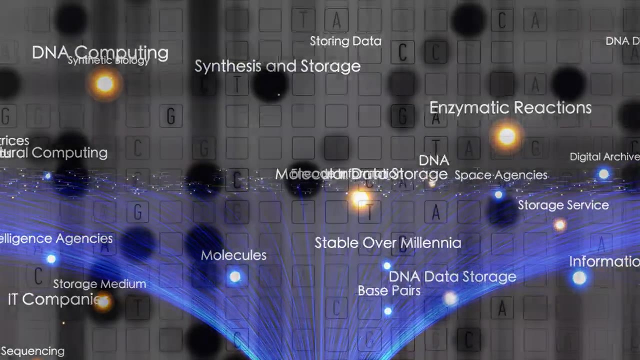 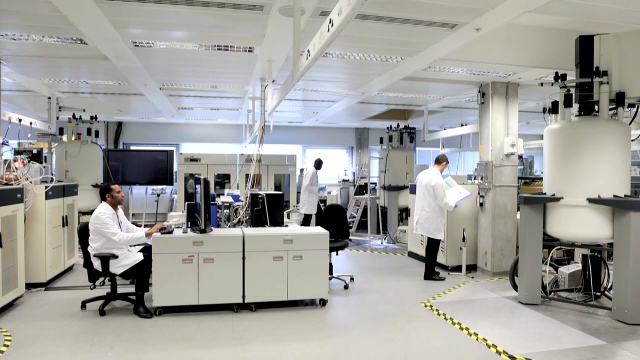 the most satisfying about all of this, about working in high performance computing- is that it supports high performance research, And so we have the great opportunity and benefit of seeing direct outcomes from the work that we do in supporting the researchers in the in their effort to make other people's lives better. But when people hear high performance, 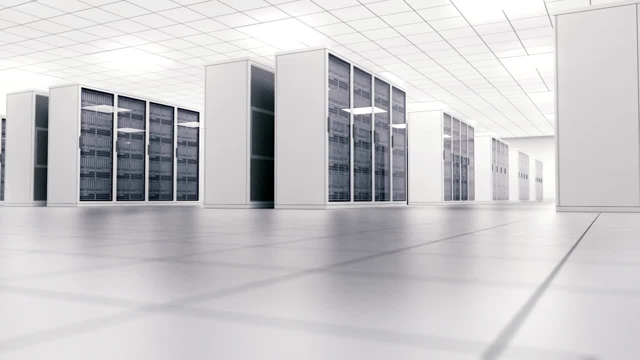 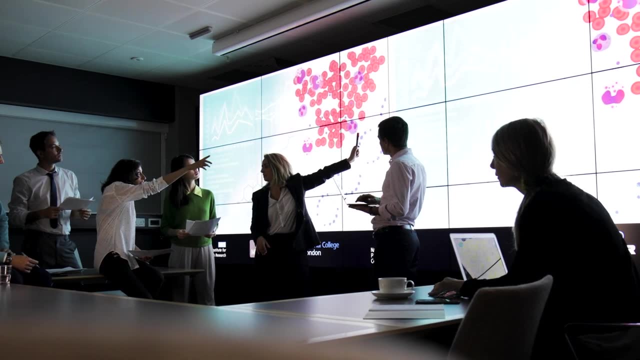 computing, it sounds, they immediately gravitate toward. oh, that means supercomputers. High performance computing is really much more simple than that. It's actually a capability, not a thing. And let me put it in terms that potentially humanize it, So that if we think 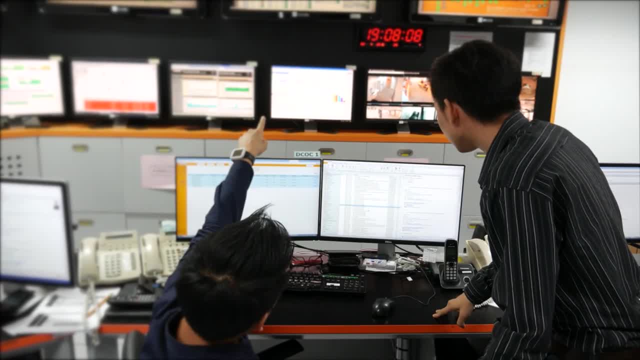 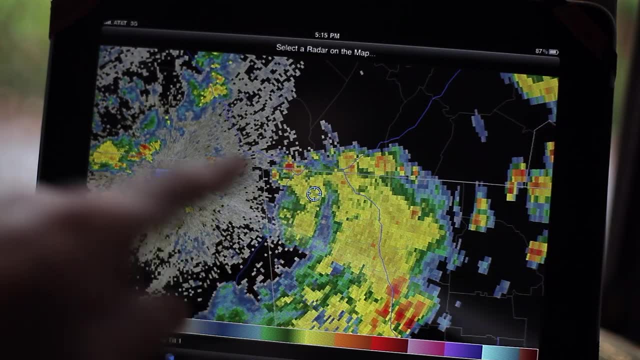 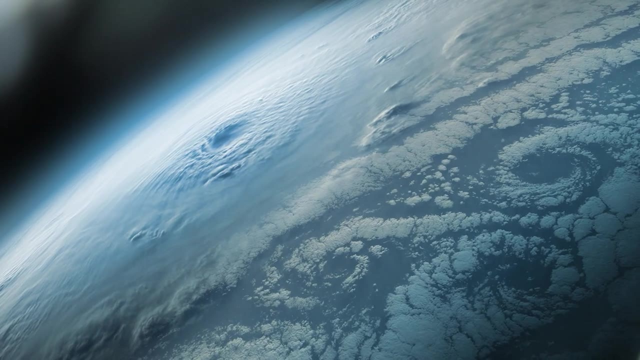 about what high performance computing is. a good example of it is forecasting the weather. There are two elements of forecasting the weather. There's getting the forecast right, writing the piece of software that takes all of the inputs and comes out with a forecast that's accurate enough so that we can make plans based off of that forecast. But there's 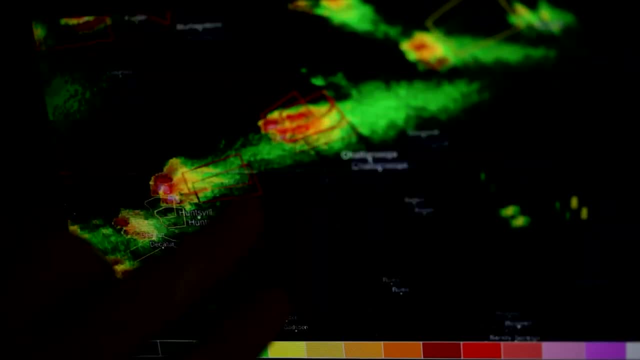 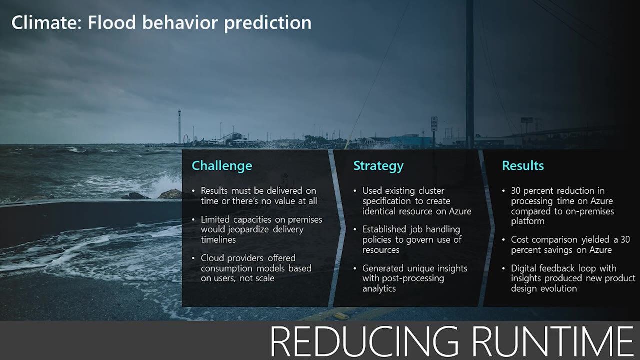 another element of it. We need to be able to run that model and get the results back in time frames that are meaningful- meaning we want to get 100 percent accurate forecast. but if it takes five days, that doesn't help us tomorrow. So the optimal situation is to 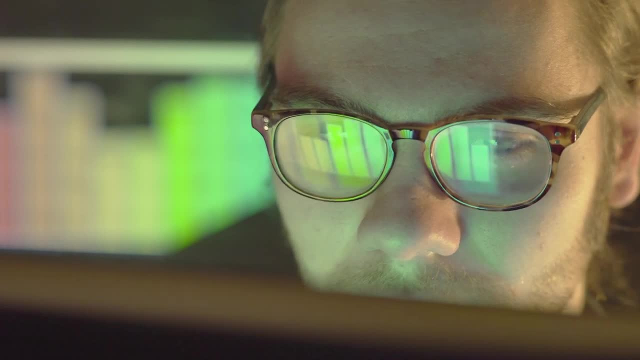 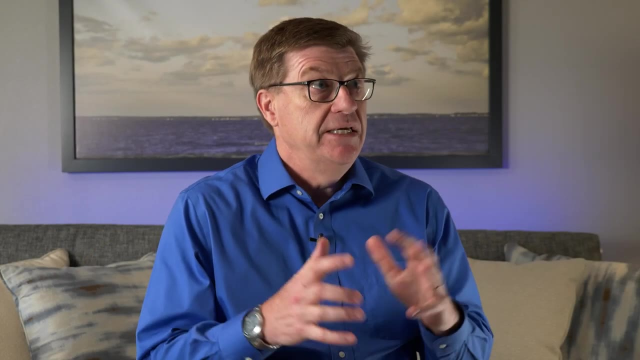 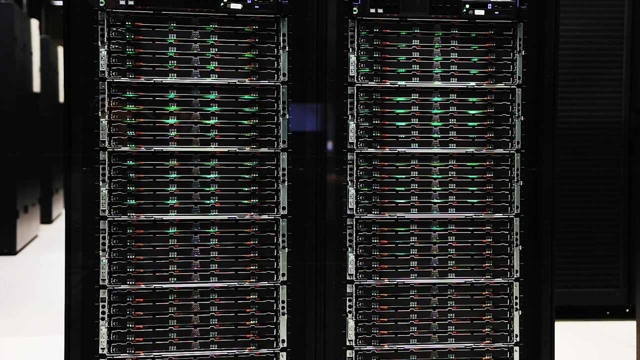 get 100 percent accurate forecast, but that we get it by tonight so that we can make plans for tomorrow. So frequently when people hear high performance computing, they immediately visualize huge rooms of blinking lights and smoked glass and cables everywhere. In actuality, 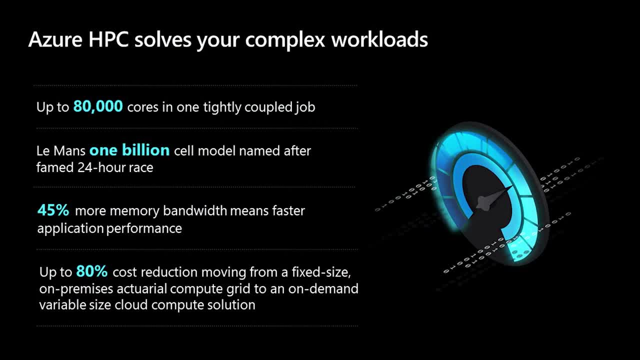 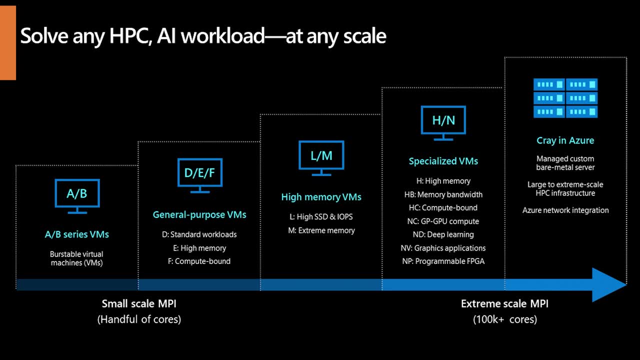 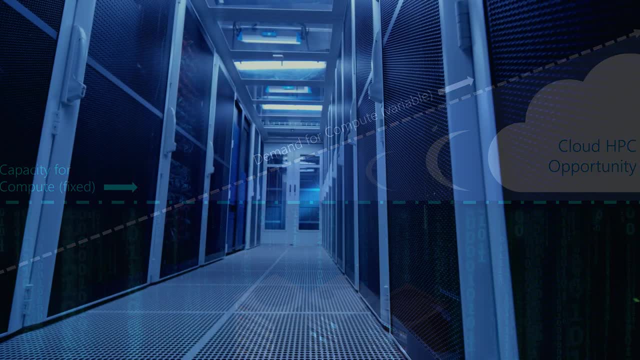 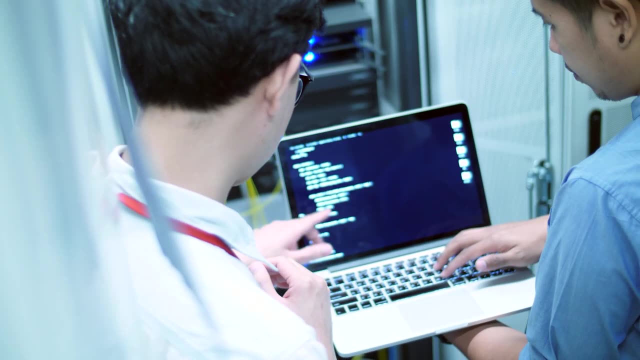 Think of HPC as the inverse of that system. What we're actually doing is taking five or 15, or 50, or 5,000 computers, using a piece of software that enables us to pull that compute resource together so that we can tackle problems that people 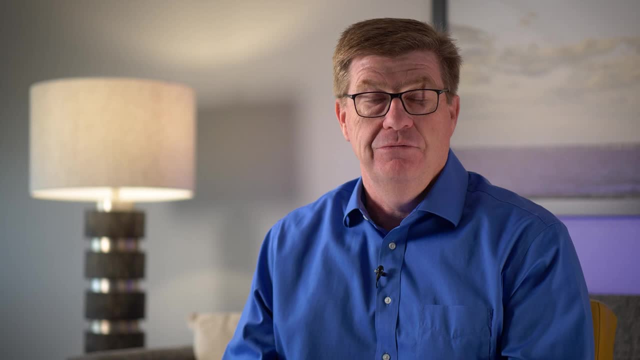 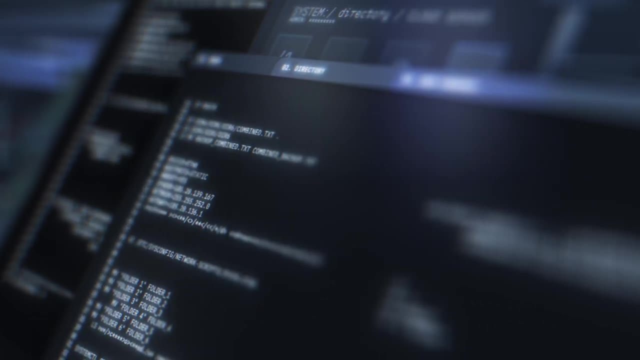 could barely imagine 50 years ago, 100 years ago, five years ago. I often use weather and weather codes as an example of not only capability but how HPC is used, because weather is one of the most taxing models and workflows in the world. 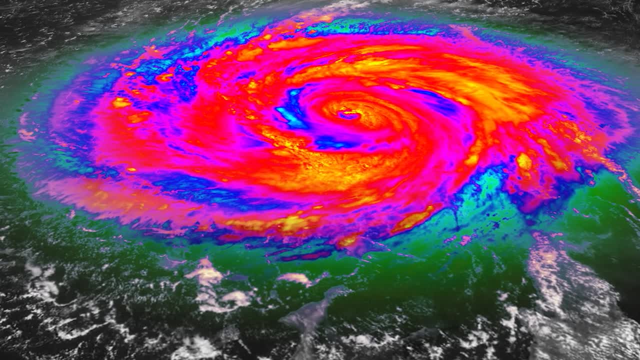 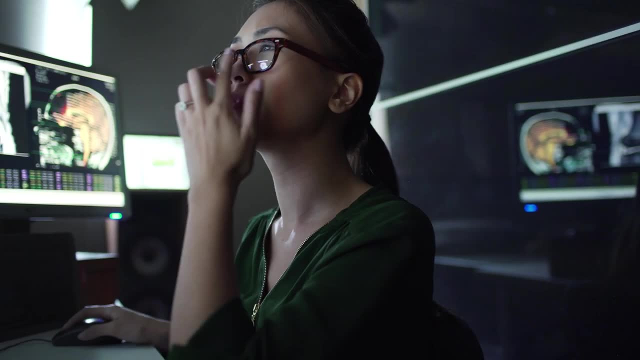 that people can run. There are a large number of inputs and it's very computationally intense, And so it's a good indicator of what's possible on a system if you can run a weather code efficiently. There is an open source weather model called WARF. 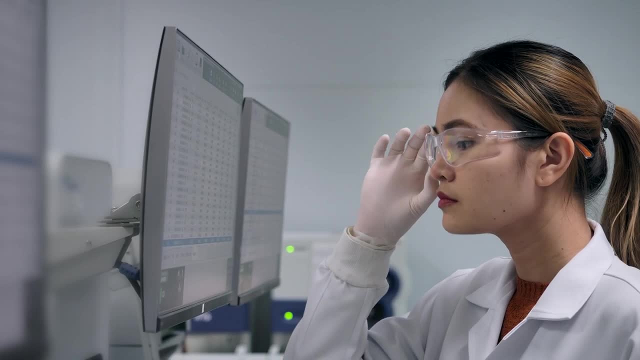 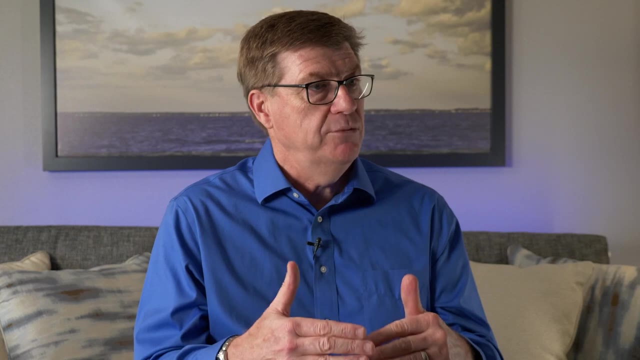 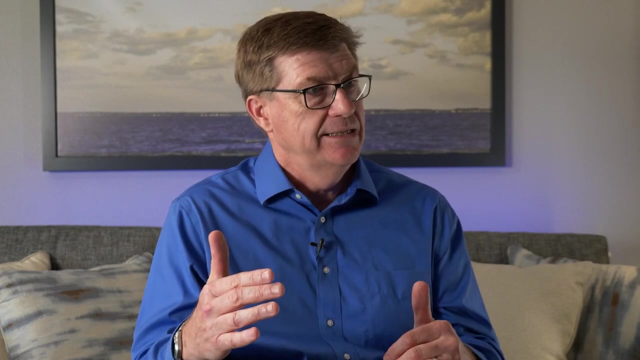 and that's used by a community of about 40,000 people worldwide who not only use it but contribute back to the code. Recently, we ran a benchmark where we were able to scale, meaning we were able to run WARF over 100,000 cores simultaneously. 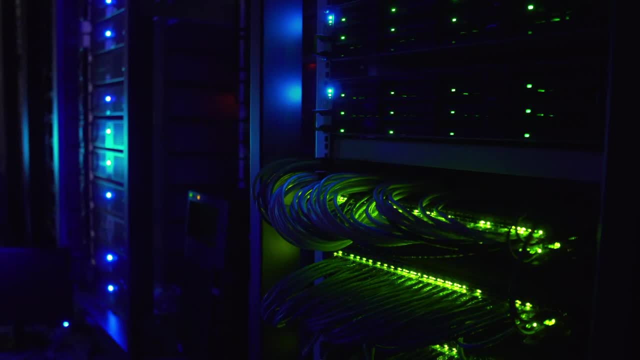 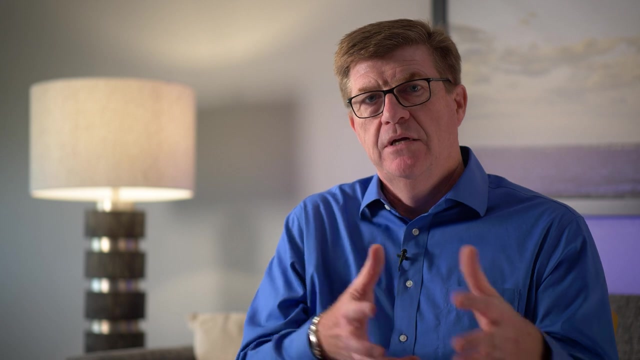 Now there are very few centers worldwide with an on-premises supercomputer with the ability to allocate 100,000 cores to WARF. But what's significant about what we did was not that we were able to run this very large workflow compared to how someone would do it on-prem. 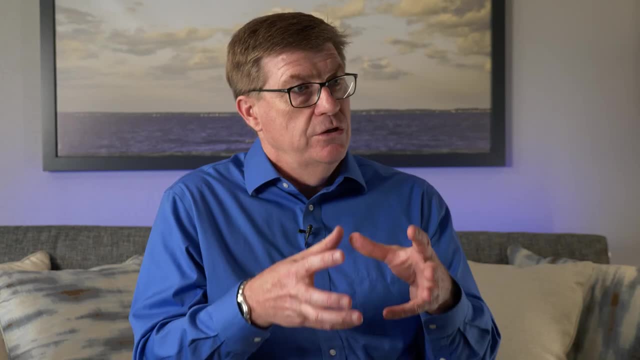 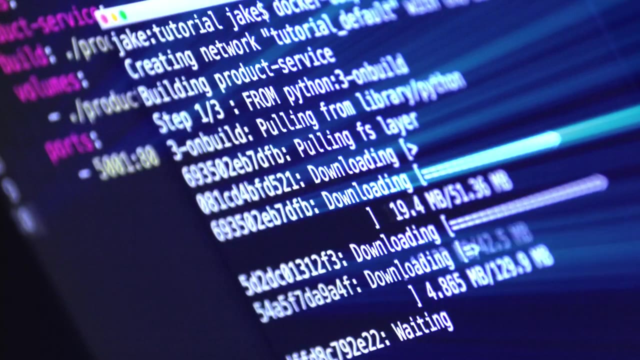 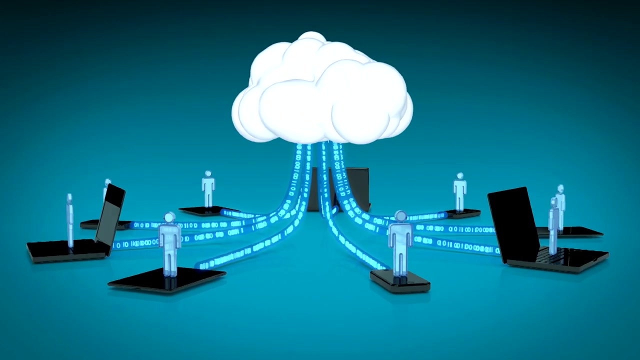 What was very important is that what we did could be replicated, if someone wanted to, by any of the 40,000 users across the WARF community. Microsoft is delivering the infrastructure and tools to the global research community to uncap their creativity and their capability.